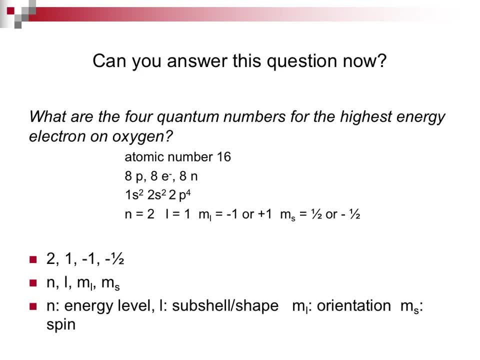 I thought a good way to teach this online was to pose: can you answer this question now? What are the four quantum numbers for the highest energy electron on oxygen atom? So if you're new to this, these are the steps you should take. Well, oxygen has an atomic number 16.. I learned 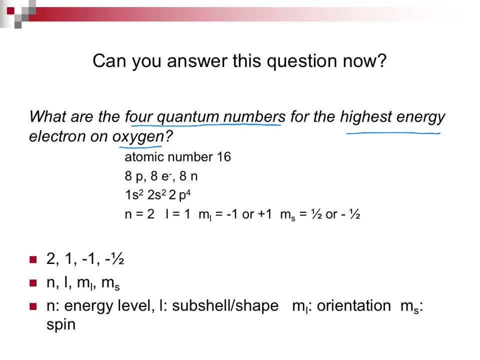 it has eight protons, eight electrons, eight neutrons. I'm going to be learning how to write the electron configuration, And what this section will then be able to do is let me take an electron configuration and turn it into those quantum numbers. Okay, don't know where you are, we shall. 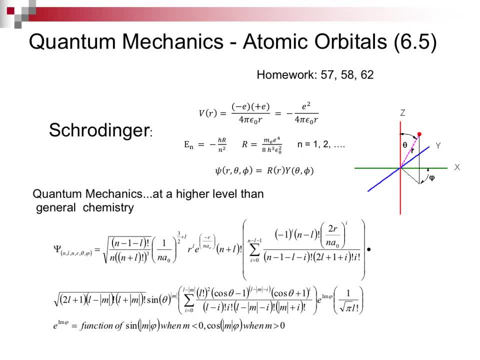 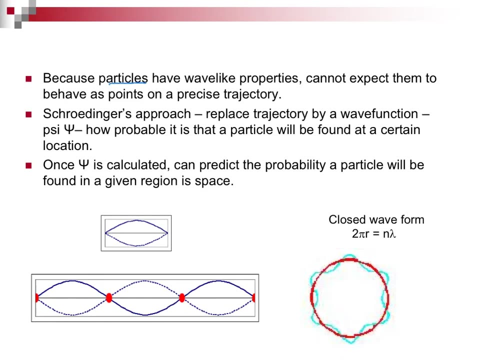 see. So quantum mechanics is atomic orbitals, and that's section 6.5.. This is not where we are going to be, because this is the heavy duty things that I learned in graduate school. Where we are going to be is trying to just get an idea of what's going on. We know that particles have wave-like 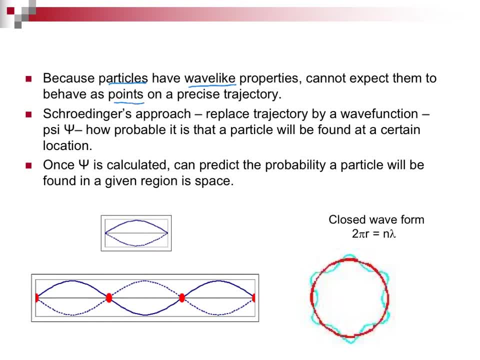 properties, but we can't expect them to behave like points. That's what Schrodinger thought He said. So once he calculated his size, he could then predict the probability of a particle in a given region of space. So what I just have here is one wave. Here I have three waves, And what Schrodinger 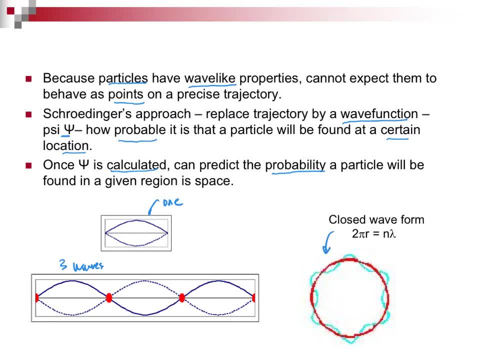 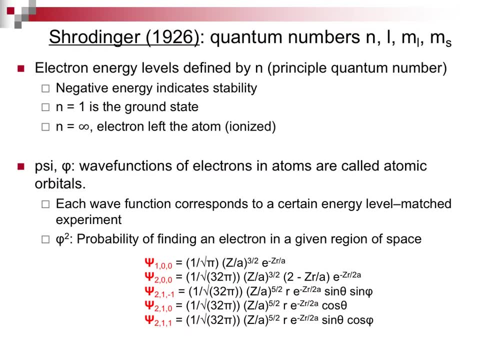 did is? he studied things and he made them into what is called a closed waveform which, in three dimensions, allowed him to predict where an electron might be. So he is the person who came up with all the four quantum numbers. So let's take it point by point. He said energy levels. 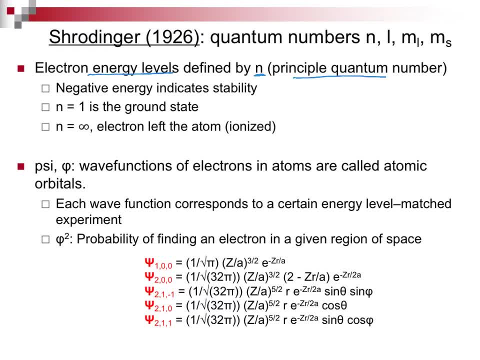 are defined by n and he called it the principal quantum number, A negative energy. that's going to indicate stability, just like it did in chapter five. He said: if n is equal to one, he's going to call that the ground state, And if n is equal to infinity, that means the 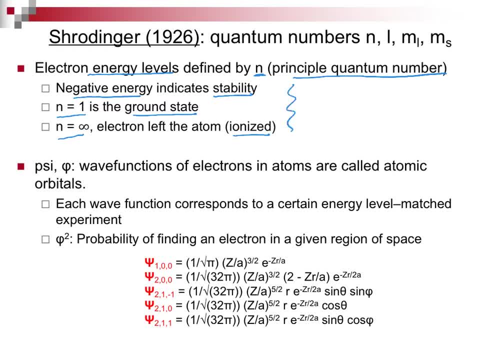 electron has left it as ionized. A lot of that comes from what we learned about with Bohr. But Schrodinger added the wave function and he called these wave functions atomic orbitals. Each function corresponds to a certain energy level and the most amazing thing is: 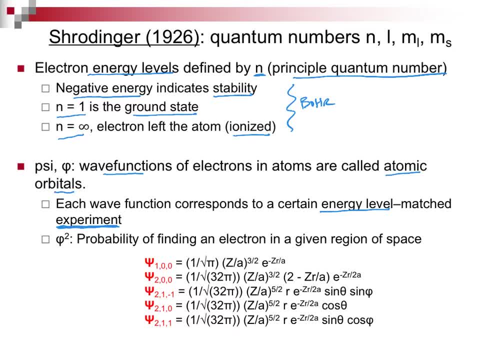 is they matched experiment. You know we've calculated wavelengths, We can get energies and frequencies. All of this came together. So if I take one of his wave functions and you see those little numbers, the one is an n, the zero is an l and the second zero is an ml. 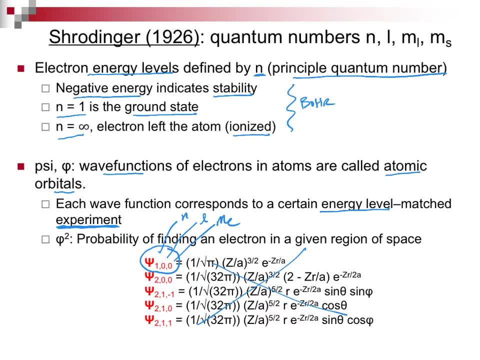 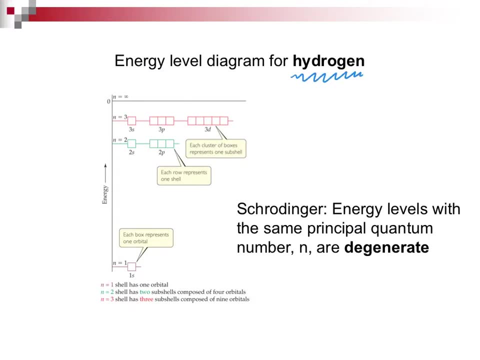 you will never have to work with these, But I wanted to show you what the meaning is at a higher level, And when you square that wave function, that's where you're going to get a probability of finding an electron. So what do we have? Well, I want to point out that this is the energy level. 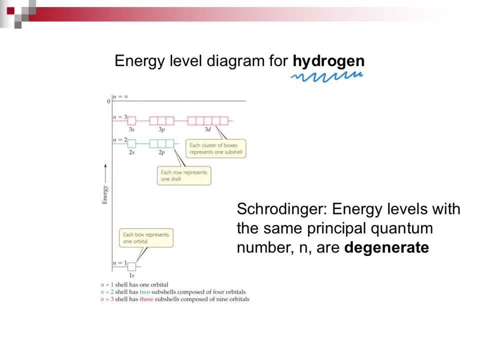 for hydrogen. only Schrodinger said. I have an energy level with the same principal quantum number, n. They were degenerate And by that we mean they have the same energy. So since n equals three, has many of them. notice how this is drawn. There's three different sets, but notice they all come at the exact same. 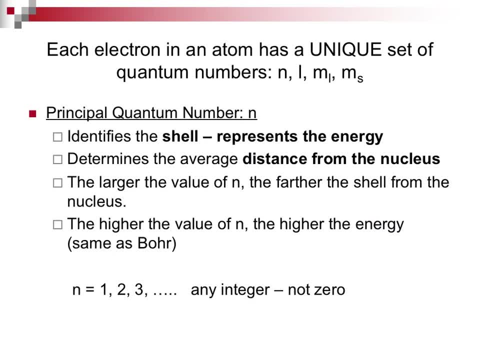 energy level. All right, Now what we're going to do is talk about each of the quantum numbers. Every electron in an atom has a set of quantum numbers. We'll cover that as we finish up the chapter, but now we introduce it. 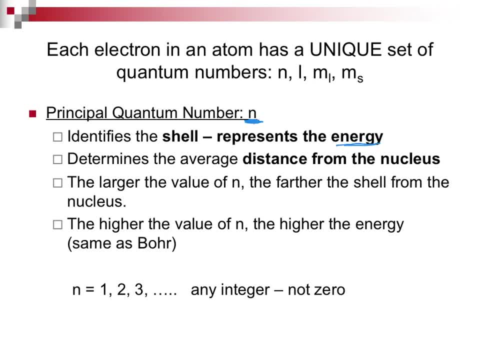 The principal quantum number is n and that represents the energy. Think back to the slide before where we had n equals one, two, three. They were further from the ground state And again it represents the average distance from the nucleus. The larger the value of n, the farther. 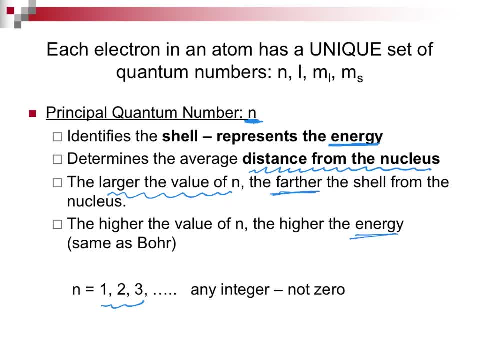 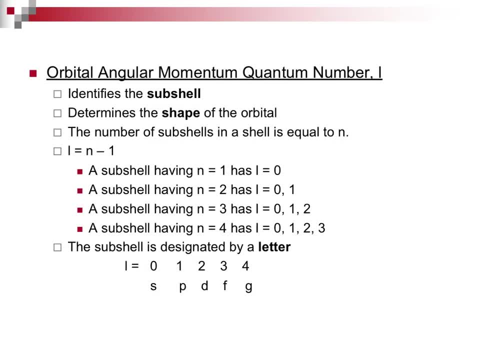 the shell will be from the nucleus And that will also give us the energy level. So we're going to a higher energy. So quantum number n- pretty straightforward. I never get much pushback on that one. The one where people start to ask questions is the one with a long name There. 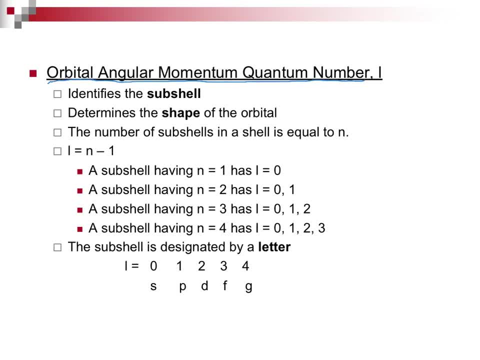 is an orbital angular momentum quantum number. It is symbolized by the letter L and it defines what is called a subshell. It will determine the shape of the orbital and your textbook breaks shape into another section. I will cover that in the next video. 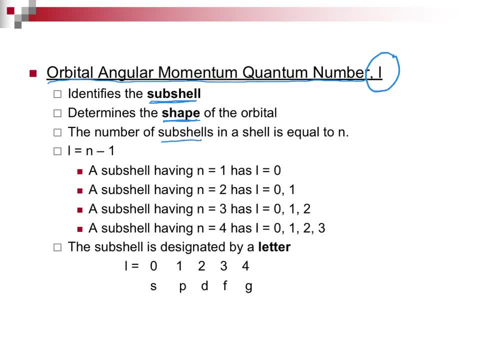 But the number of subshells is equal to n and L is equal to n minus one. So if I have an n of one, I will have a number, an L, equal to zero. If I have a subshell with an n equal two, my L will now be: 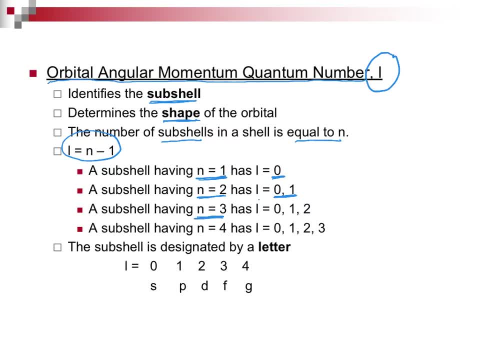 both a zero and a one. If I have an n equal to three, it will be a zero, a one and a two and n equal four. A zero, one, two, three. Now you may say: why did I do all those four examples? Because people. 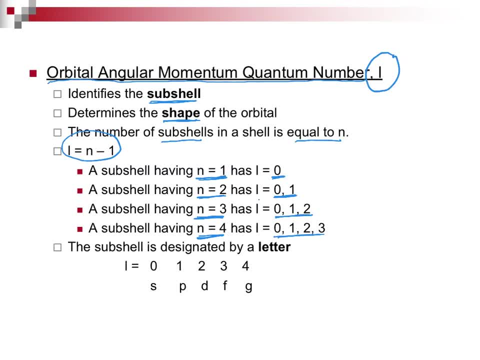 really struggle with this. This is quantum chemistry. all right, To top it off, every time I have a subshell, it's designated by a letter. If I have a zero, it's an S, If I have a one, it's a P, If I have a two it's a D, and on and on. Each of these has a specific shape, that is. 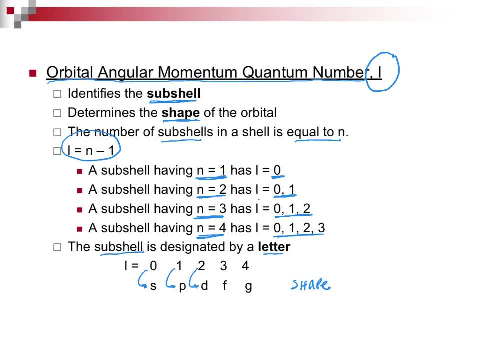 covered in the next section, But for now we want to say L represents the subshell, the subshell represents the shape and the number of subshells is equal to n. Notice for an. n equals two. we have two subshells. 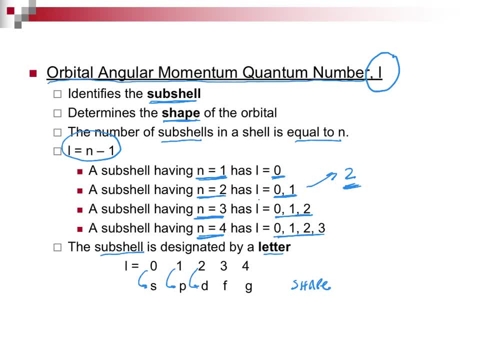 In order for me to determine the actual quantum number, what I will do is I will subtract one. So let's say we have a five, an n equals five, The L will be zero. one, two, three, four. Those are the rules. They came from the wave functions that Schrodinger 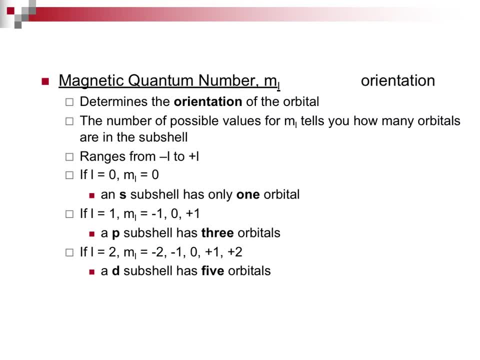 developed all right Magnetic quantum number. that is not quite as bad. A magnetic quantum number tells us it's designated by an M with a subscript L and we're going to see in the next section how it is an orientation. The number of possible values tells me how many orbitals are. 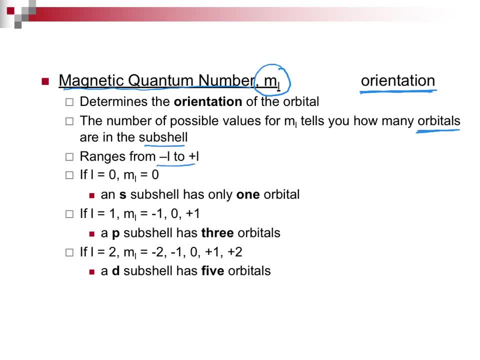 inside a subshell. So we're going to see how many orbitals are inside a subshell and we're going to a subshell and it ranges from minus L to plus L. I've given the three that we're going to encounter in this class. If I have an L equals zero, that will make my ML equal to zero. That 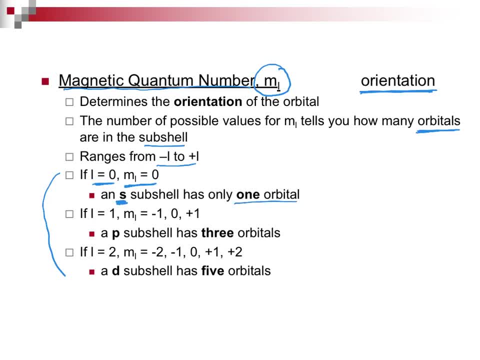 represents an S subshell and there's only one orbital. I usually will draw it with a line and put a little S underneath. If I have an L equals one, my ML will range from minus L to plus L. So I will have three of these orbitals. We'll have a designation, minus one, zero plus one. These are: 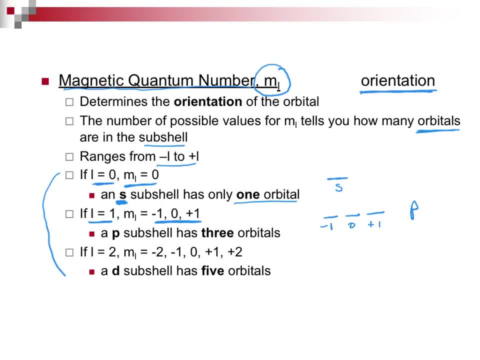 the Ps and at our level, we don't worry about how we exactly label it. We only know that there's a minus one, a zero and a plus one. So the third one we're going to encounter in this class is an L. 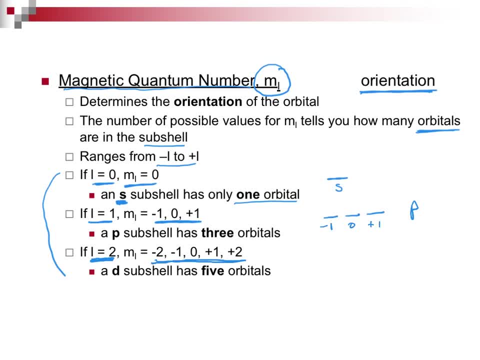 equals two, where the ML is equal to zero. So we're going to have a designation minus one zero plus one. So we're going to have a designation of two minus two, minus one zero and plus one. If you've done. 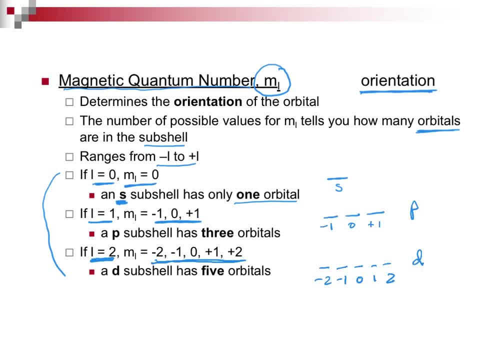 this in high school. you probably know where this is going, but essentially we will be writing the electron configuration for elements in the periodic table. So the things to point out here are: L equals zero is an S. There is one orbital. If L equals one, it is a P, and that is three orbitals. If L equals two, it is an S. There is one orbital. If L equals one, it is two orbitals. If L equals one, it is a P, and that is three orbitals. If L equals one, it is a P, and that is one orbital. 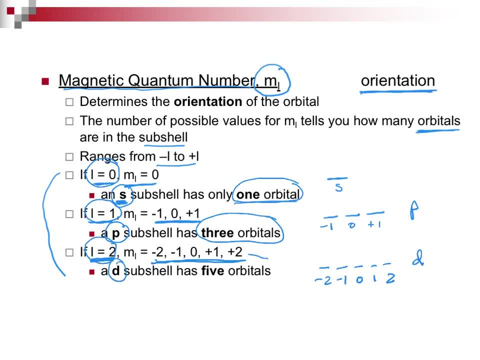 L equals 2, that is a D and that is 5 orbitals. For those of you seeing it for the first time, it's pretty hard to wrap your head around, but this is what it is: an N, an L and an ML. 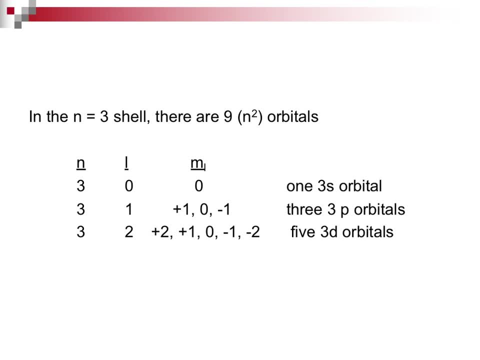 In each of them. what did I do to finish this section? Well, I know the struggles many people have, So what I did is I said: let's say I have an N equals 3.. As you can see, my values of L are 0,, 1, and 2.. 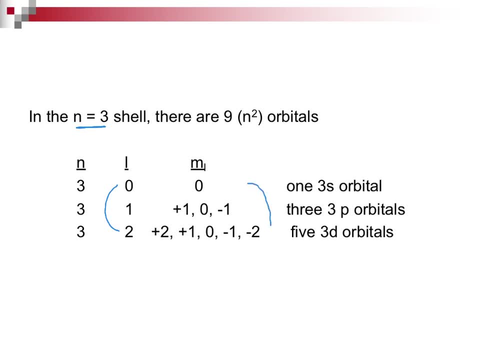 As you can see, my values of ML are: 0 for L equals 0, plus 1, 0, minus 1 for L equals 1, plus 2, plus 1, 0, minus 1, minus 2 for L equals 2..